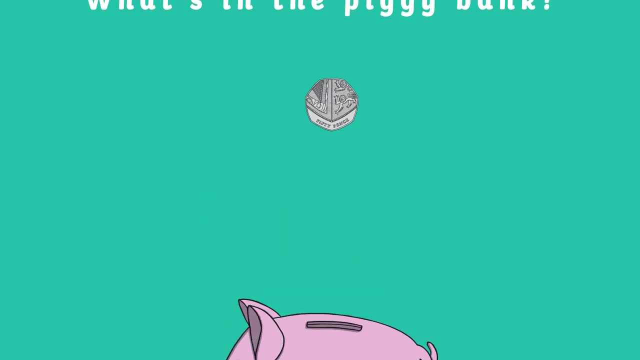 If you add 5p to the next coin, it's 10p. If you add 5p to the next coin, it's 10p. If you add 5p to the next coin, it's 10p. 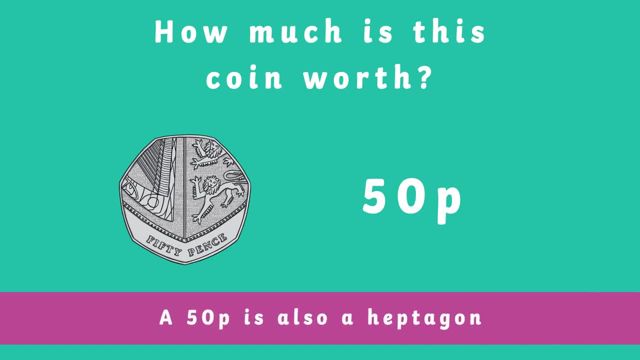 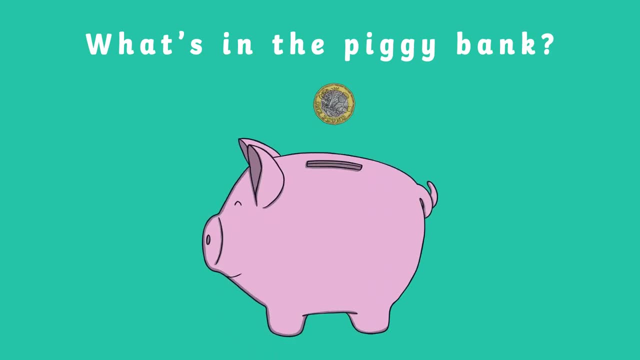 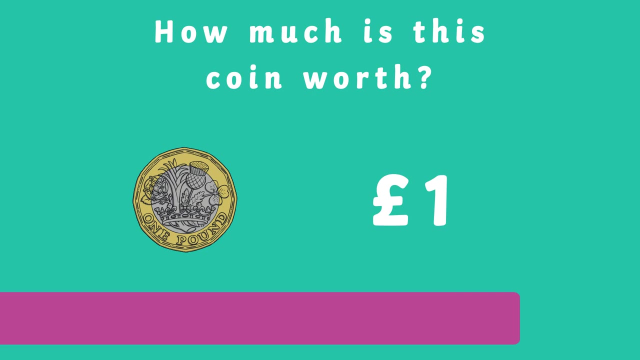 Did you know that a 50p is actually the shape of a heptagon? Next up is our 1£ coin. Next up is our 1£ coin. We use the pound sign to represent this coin. We use the pound sign to represent this coin. 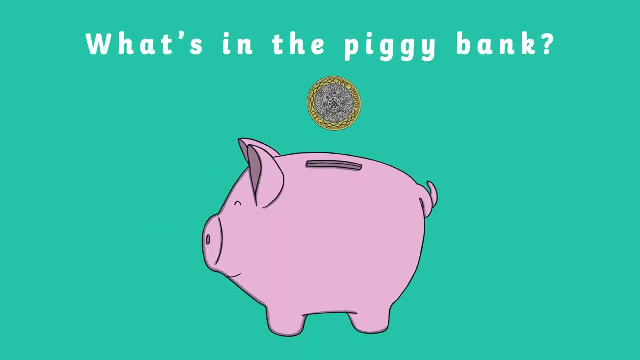 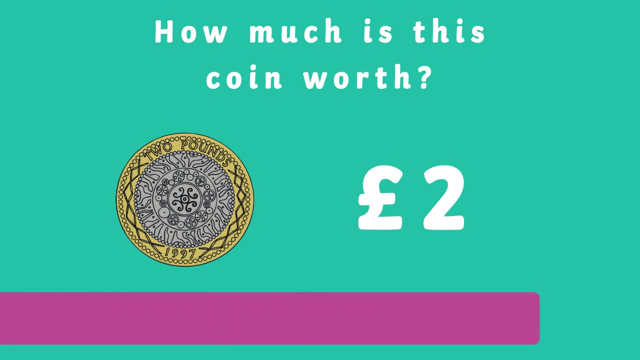 Our last coin is called two pound. Two hundred 1p's are worth the same as two pound, so we still use the pound sign when writing this coin. 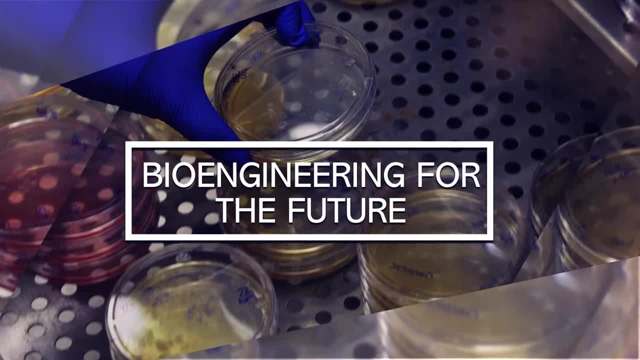 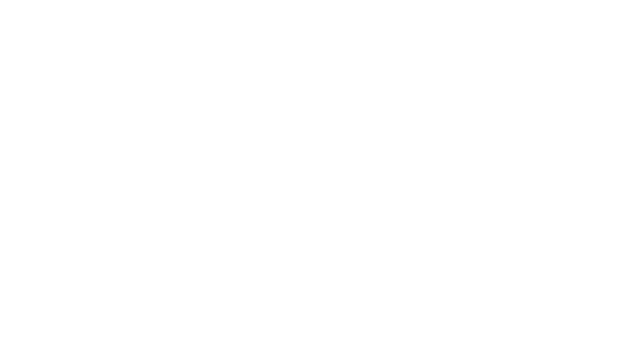 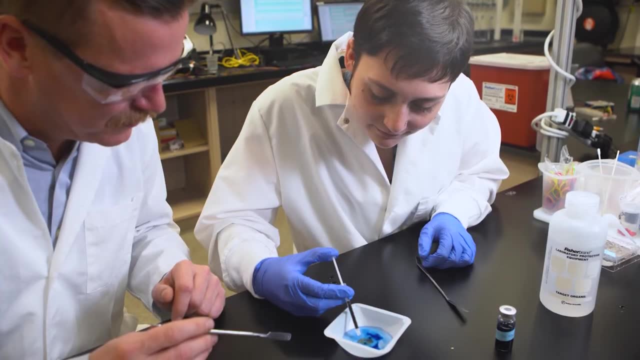 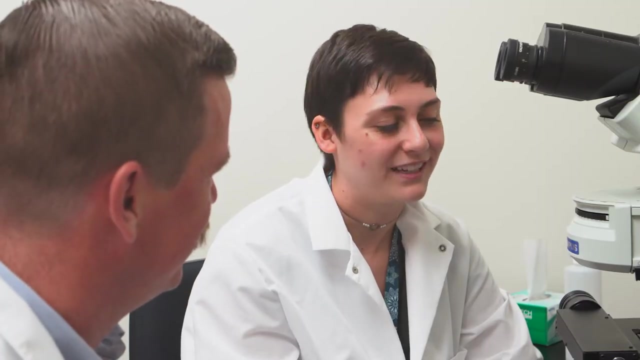 Pulmonary biomechanics is the relationship between pressure, volume and flow of the pulmonary system, And this arises from the structure of the lungs and the chest wall and is supplemented by the important surface tension forces in the lung and pulmonary surfactant, which play a major role in the stiffness of the lung as it's inflated. Thank you for watching.